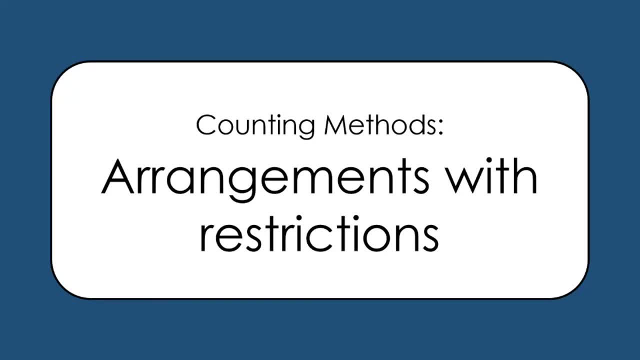 Okay, so here we're going to look at arrangements involving restrictions, and really students tend to find these problems quite hard because there's no one way to go about answering any one of these questions. It's really just about stopping and thinking. quite logically, A pigeon-holing technique is really useful in these sorts of problems in many cases. So let's get straight into some examples. 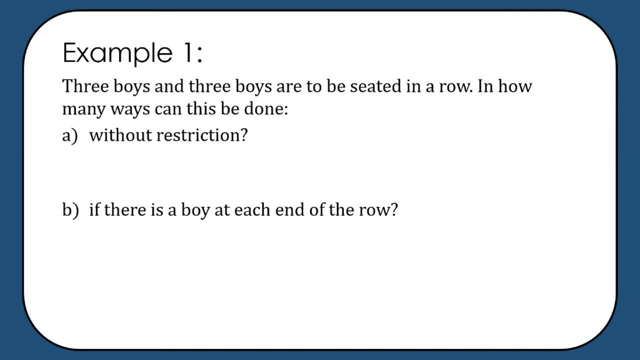 So we have three boys and three girls that are to be seated in a row. In how many ways can this be done without restriction? So if there's no restrictions on how the three boys and three girls can be seated, we essentially just have six people that need to be seated in a row. So we know from our previous video that there are six factorial ways that that can be done, And six factorial is 720 different ways that these girls and boys can sit in a row. 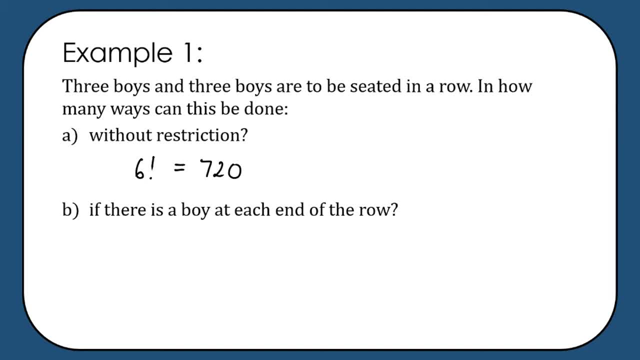 Okay, then in how many ways can it be done if there is a boy at each end of the row? Okay, so if we think about the fact that we're going to have six people seated in a row and we need to have a boy at each end, A boy and a boy. 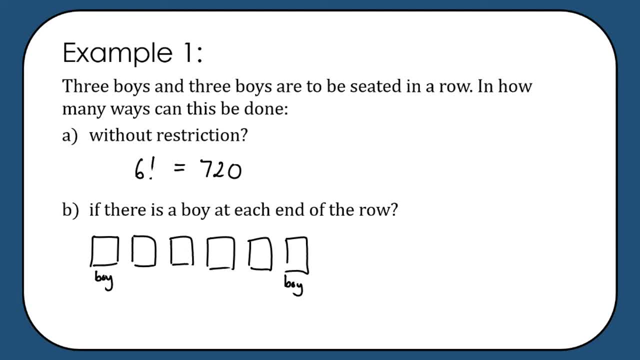 So whenever you're dealing with problems involving restrictions, you want to think about dealing with the restriction first and then working out how everyone else is going to fit around it. So we need to put a boy in the first position, and there are three boys to choose from. 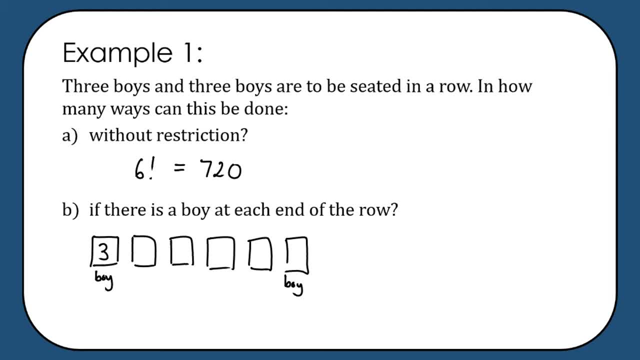 So there are three boys to choose from and there are three boys to choose from. So there are three boys to choose from and there are three boys to choose from. So there are three different options that could go here. Then, once we've put a boy in the first position, we also need another boy in the last position. 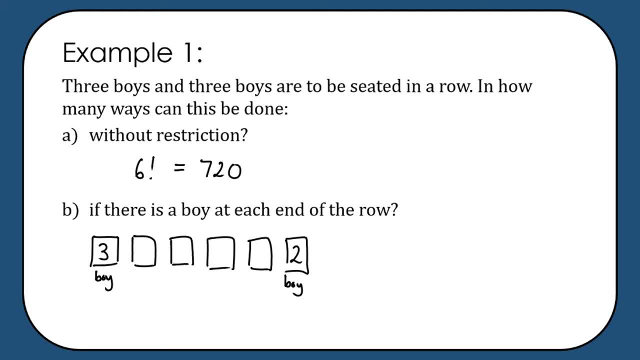 So there's two remaining boys to choose from to go here. Now there's no restriction on how these four people in the middle here are going to be seated, And so there's simply going to be four factorial ways that we can arrange them. Again, we need someone in every seat. 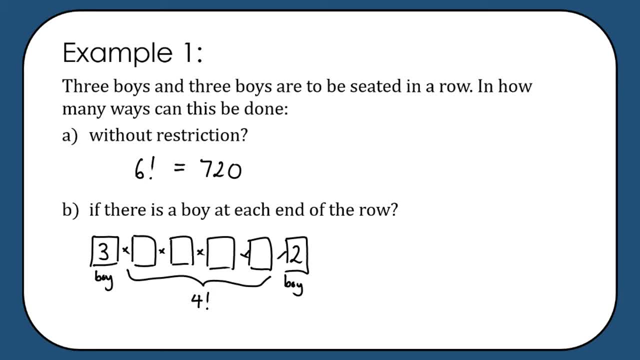 So this is a multiplication situation. So we have three times four factorial times two Different ways that we can arrange the girls and boys. So that comes to 144 different possible arrangements. Same problem: Three boys and three girls are to be seated in a row. 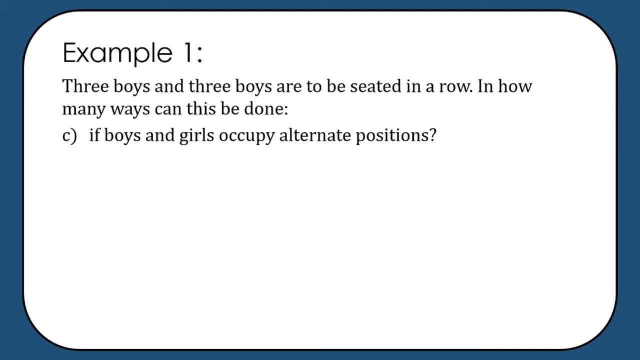 In how many ways can this be done if boys and girls occupy alternate positions? Okay, so there's sort of two ways to think about this kind of problem. Okay, so the first is Alright. again, in both cases, we're going to think about our six positions. 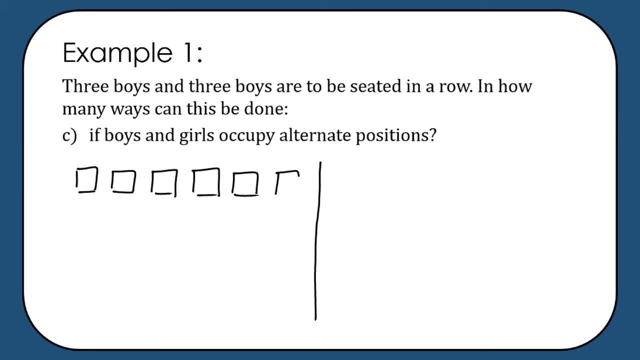 and how we might logically think that through. So we've got six positions And we need to alternate. So we need those three people to be- let's say: Oh sorry, not those three, Let's fix that. Those three people to be, let's say, girls. 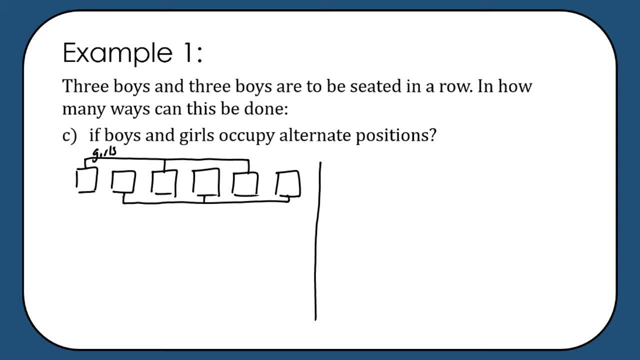 And we need those three people to be boys. So there are three factorial different ways that we can arrange the three girls and three factorial different ways that we can arrange the three boys. Now there's one other thing that we haven't thought about in this situation. 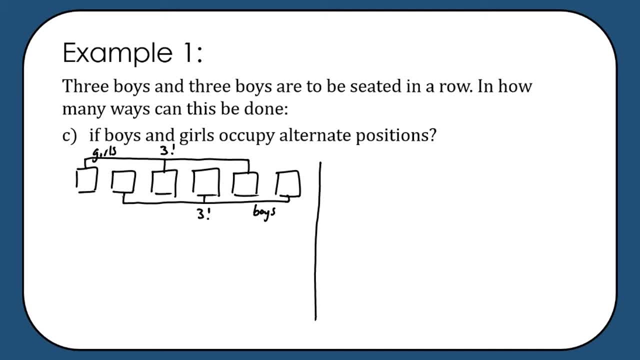 because we've assumed that we're going to start with a girl. So obviously we could have this exact same situation, but instead starting with a boy. So there's going to be two different ways. We're going to multiply our options by two, because that would be when we start with a boy instead. 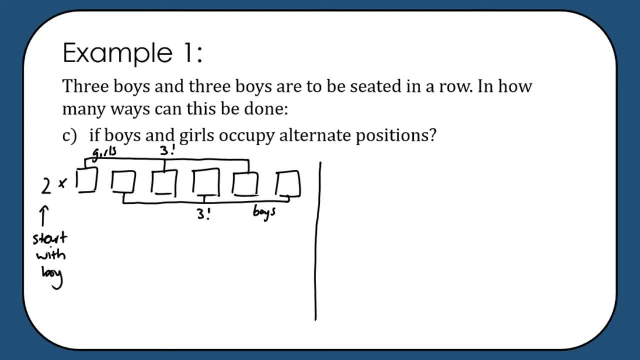 So, starting with a girl, there'd be three factorial times three factorial different ways for that to happen. Starting with a boy, there'd be three factorial times three factorial different ways for that to happen. So we have two times three factorial times three factorial. 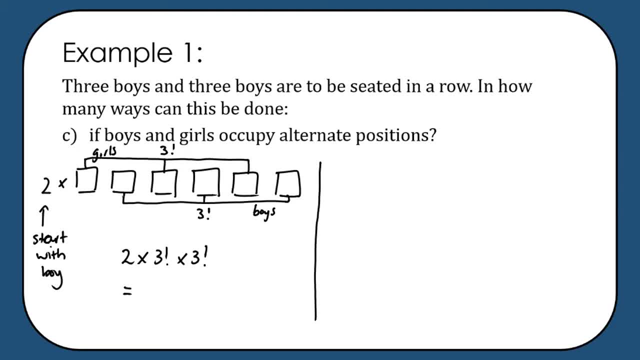 We know three. factorial is six, so that's two times six times six, So 72 different ways. The other way we can think about it is again thinking about our little pigeonholes, and what options have we got for each one? Okay, so if we think position by position, 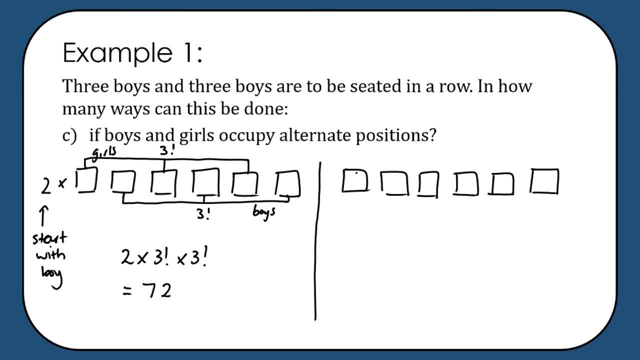 So the first position: any of the six people could sit here. Boy, girl, doesn't matter. Then in the second position, it has to be so. let's say, for example, a girl was sat in the first position, then it would have to be one of the three remaining boys in the second position. 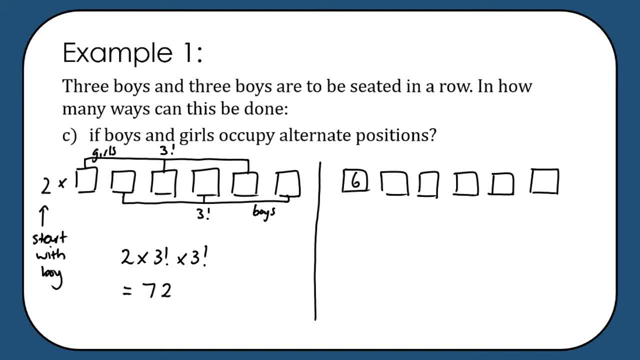 Or let's say we sat a boy in the first position, then it would have to be one of the three remaining girls in the second position. Either way, there's three different ways. So there's two different options here. for the second position. 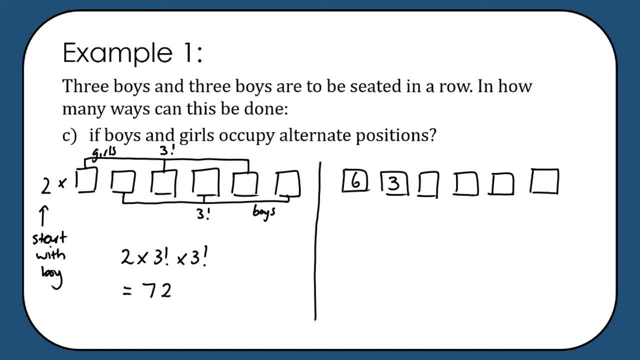 Okay, so then we've now seated one boy and one girl, So there's two different options for the next position and two different options for the next position where we need to again seat a boy and a girl. Now we've still got one girl and one boy left. 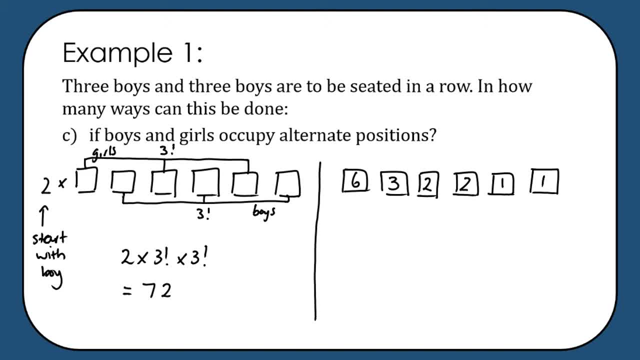 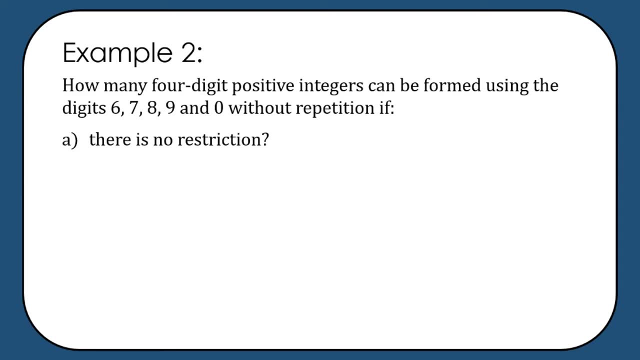 and so they're going to each go into these two positions. So we have six times three times, two times, two times one times one, which again gives us the same answer of 72. So we've got two different arrangements, Okay. example two: 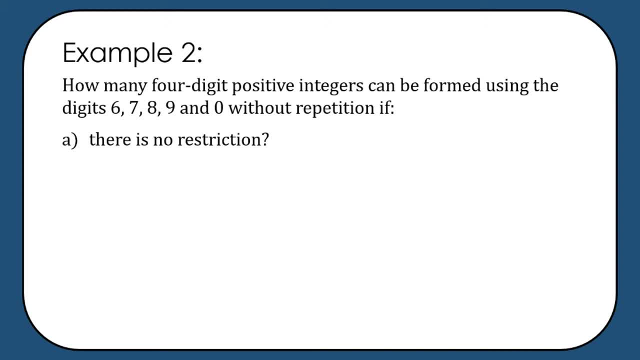 How many four digit positive integers can be formed using the digits six, seven, eight, nine and zero without repetition, if there is, first of all, no restriction? Now, these kinds of problems are fairly common. but what you need to be really, really careful about here, 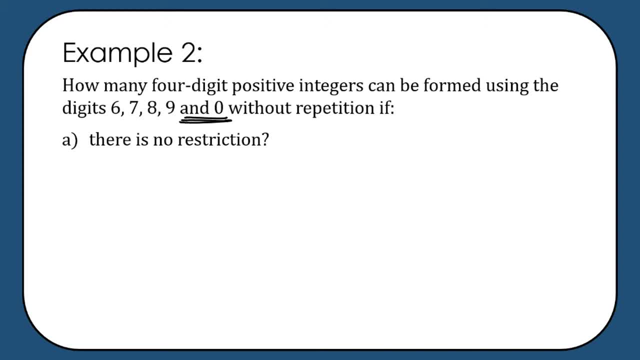 is the fact that zero is included in this set of digits that we're dealing with, because zero has its own set of restrictions implied Because we want to form a four digit number. Yes, there's no restriction, but it's not. simply we've got five digits to choose from. 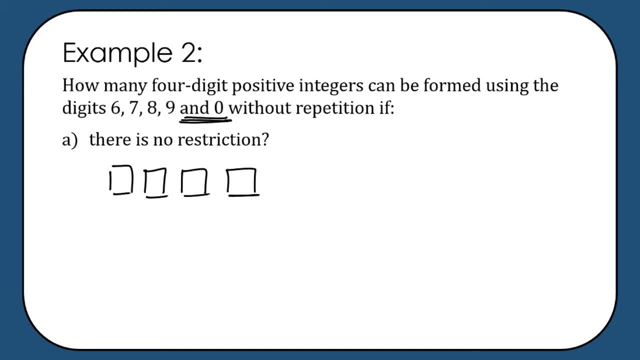 but it's not just going to be five factorial in this case, because of the zero. So if we want a four digit number, we can't have zero at the beginning. That wouldn't be a four digit number, that would be a three digit number. 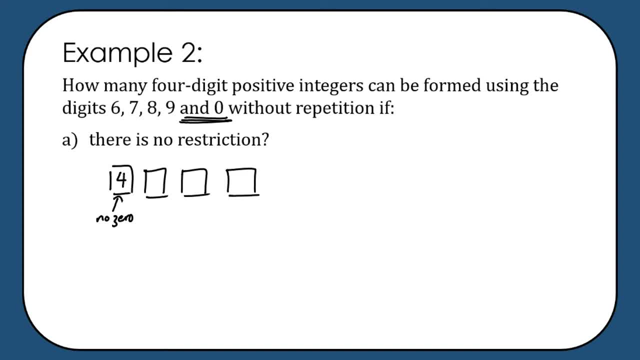 So actually it means we've only got four options for what could go at the beginning. We're creating a number without repetition, so I've put a number in the first position. I can't use that again, So, but I can use the zero now. 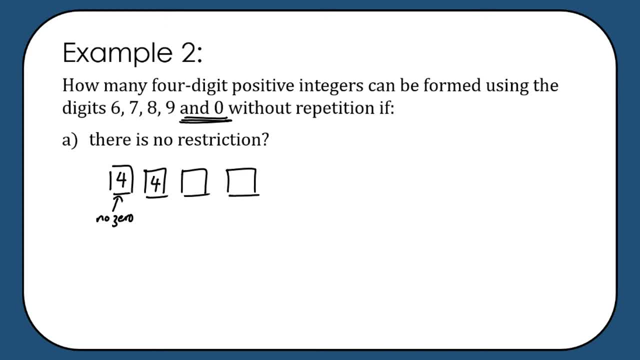 so I've got four different options. again at the second position, then I've got three options and then I've got two options. So four times four times three times two. Let's go to my calculator quickly. Four times four times three times two is 96 different options, with no restriction. 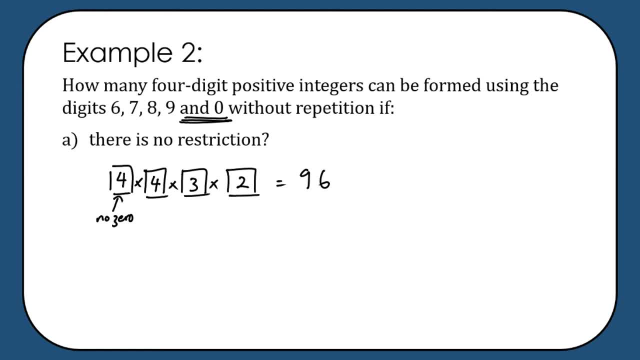 Bearing in mind that no restriction is a loose statement, given that zero itself implies some restrictions. Okay, same problem. Four digit positive integer formed using the digits six, seven, eight, nine and zero, without repetition if the number has to be greater than 8,000.. 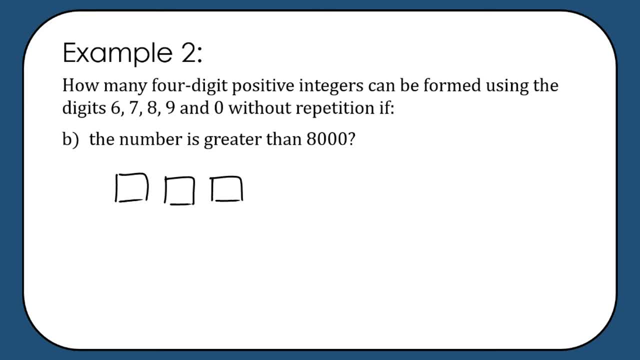 So again we want a four digit number, but here it has to be greater than 8,000.. So that means there's restrictions on here, That one can be only eight or nine. So we've only got two options to go there. 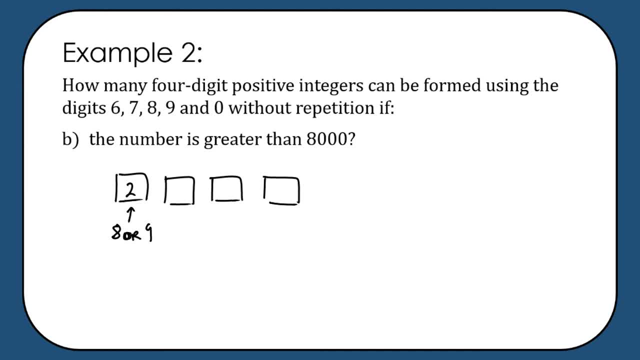 and then we completely can put anything after that. Again, it's without repetition. So we've put eight or nine in the first position. That leaves us with four different digits to choose from here: three digits to choose from here and two digits to choose from here. 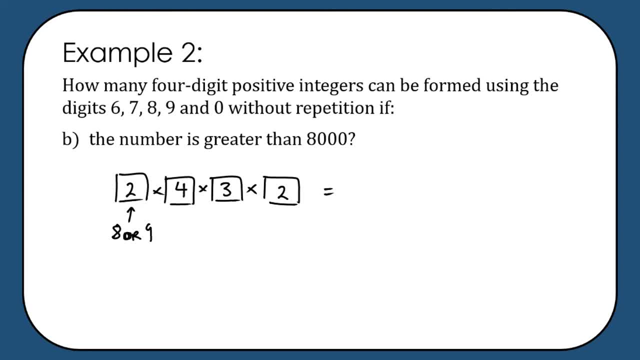 And so we've got what's that? eight times three is 24, times two is 48. different options to create a four digit number greater than 8,000.. Okay, part C, Same problem: Four digit positive integer formed using the integers six, seven, eight, nine and zero, without repetition. 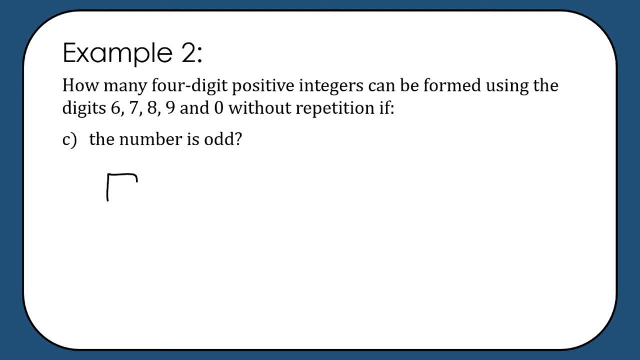 if the number is odd, Okay. so if we've got an odd number, the restriction is on here. So that means that that has to be an odd digit for the whole number to be odd. So that means that digit has to be seven or nine. 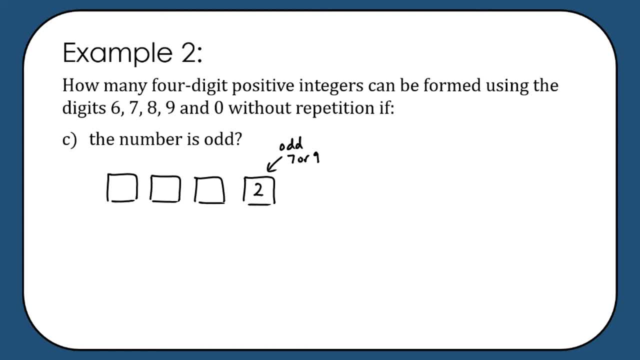 So we've got two options that can go there. Then we worry about filling in all the other spots where there aren't restrictions. Again, though, there is a restriction at the first digit, So we have four digits remaining to put in the first position. 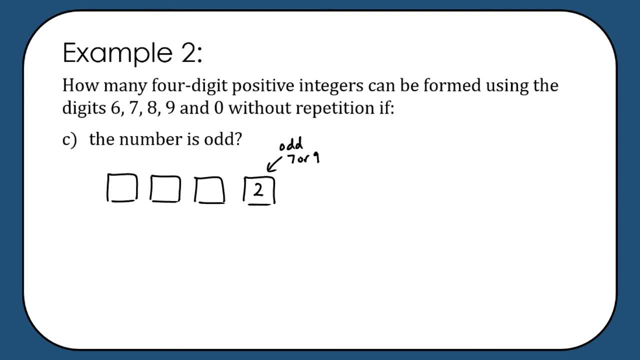 but one of those four digits is zero. So we actually only have three digits that could go in the first position. Then we've got three digits remaining. They can all go in the second position, and two digits remaining- They can all go here. 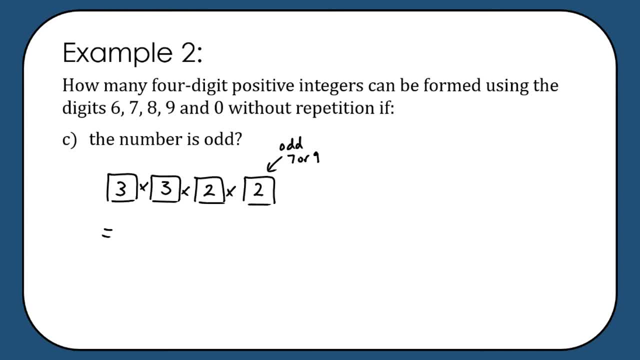 Again, we want a number in each of the four positions, So it's an AND situation. So we're multiplying three times three times two times two, It's nine times four, So 36 different options And part how many four-digit positive integers can be formed. 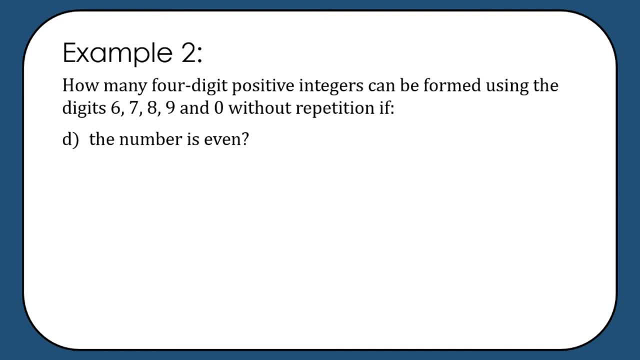 using the digits six, seven, eight, nine and zero without repetition, if the number is even Okay. so the best way to think about this is: there's a couple of different ways And we need. this can be quite a complex problem. 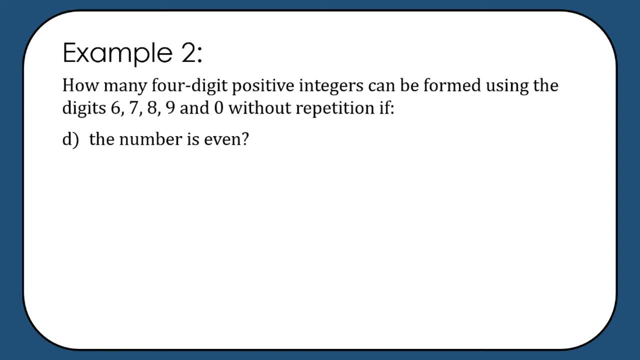 starting from scratch. Given that we've just worked out the number of options where the number is odd, we're actually quite a long way along the way to answering this problem. I'm just going to flick back here to get some of our answers we need. 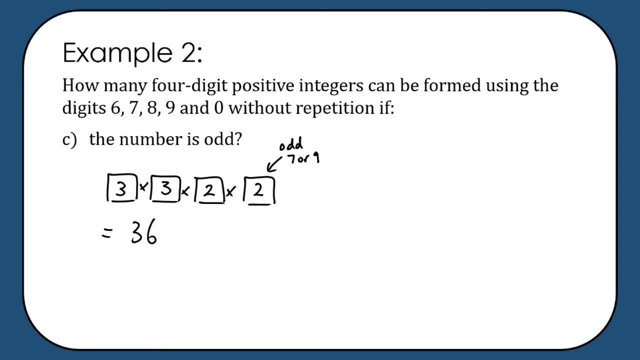 So we worked out in part that there are 36 odd numbers. In part we worked out that there are 96 numbers in total that could be created. So what we find is that there are 96 numbers. We want the total number of options minus the odd options. 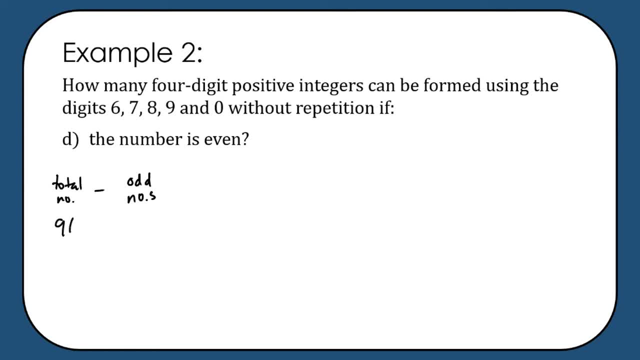 Which means it is 96 minus 36.. And so that means there must be 60 even options, So that's definitely the quickest way to go about that. If, though, we hadn't worked out the number of odd options already, then we need to think about the number of even options. 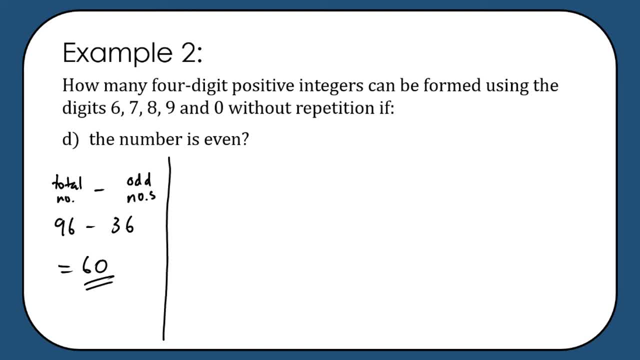 And again, the zero in this problem makes things quite difficult. We really need to think about two different cases: The situation where the number ends with a zero, which would make it even, and the situation where the number ends with six or eight, as two different things. 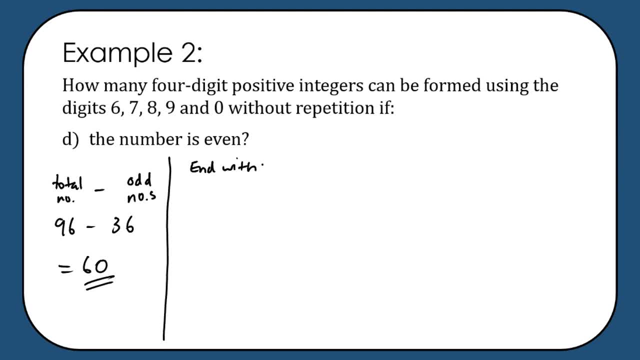 So, first of all, if we end with a zero- so we've got our four digit number- we're going to put the zero at the end, so there's one option. for the last number, The zero is already taken out of the mix. 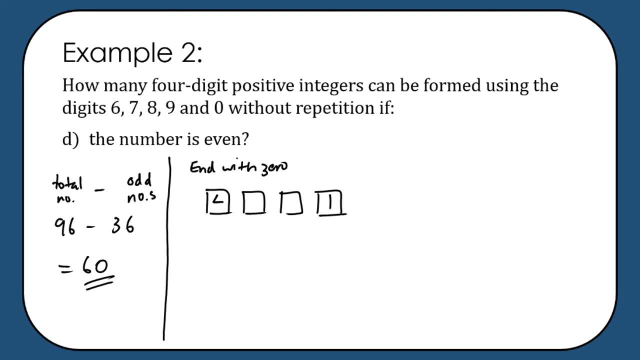 We've got four digits remaining, and any of those four digits could go at the beginning, because zero is already taken care of. Then we've got three different options here And two different options here. So there are 24 different four digit numbers that end with a zero. 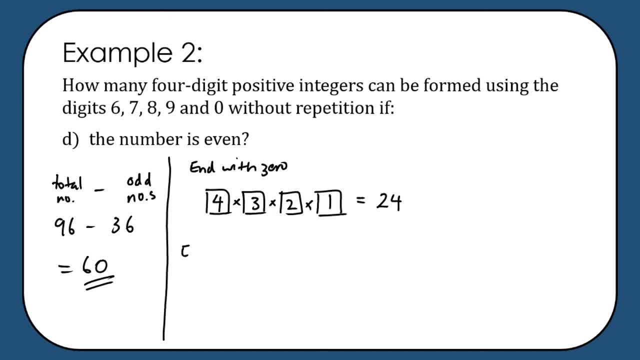 So they're all even numbers. Then we need to think about ending with the non-zero even numbers. So in this case that is six or eight. So in this situation we've got our four digit number. There are two options for what we could put here. 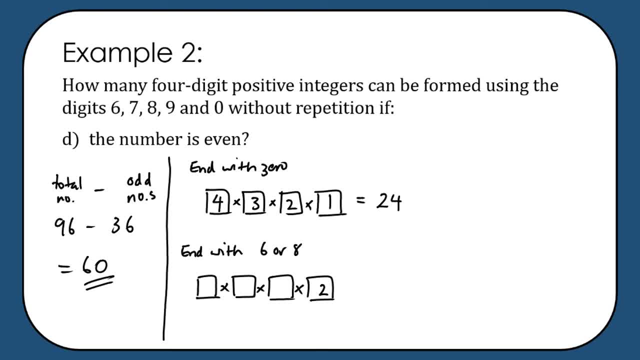 Now, this time, zero is still in the mix of the four different digits remaining, So I only have three options available for the beginning. I still have three digits remaining. Any of them could go here. Now I have two digits remaining. Two of them could go here. 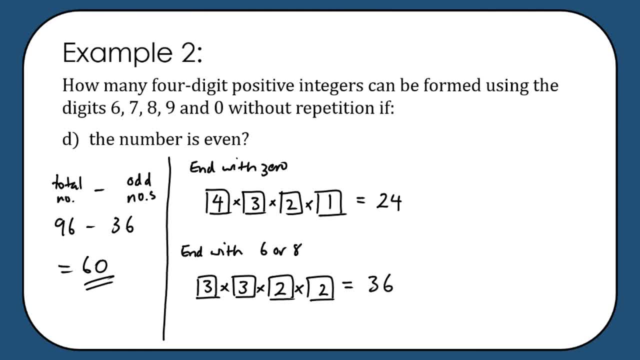 And so we've got 36 different options here. The number is either going to end with a zero or end with a six or eight, So that means that we're going to add together 24 and 36 to find that we get 60 different arrangements. 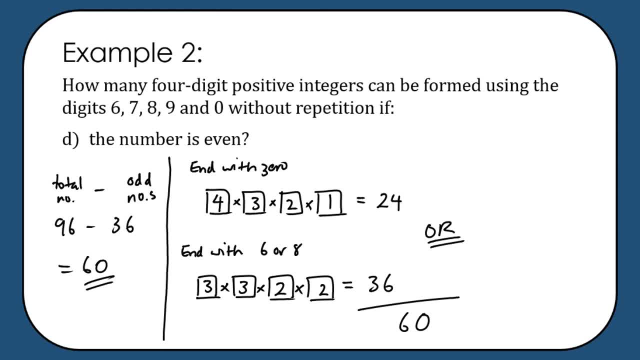 So you just need to be very careful when your example has, when your list of digits includes zero, because zero can't go at the beginning of a number if it's to be three or four digits. So you need to think quite carefully about that. 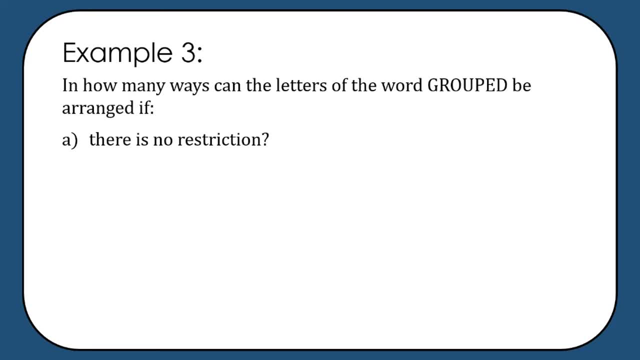 Okay. example three: In how many ways can the letters of the word grouped be arranged if there is no restriction? Okay, so we have one, two, three, four, five, seven different letters. So if there's no restriction, seven, factorial. 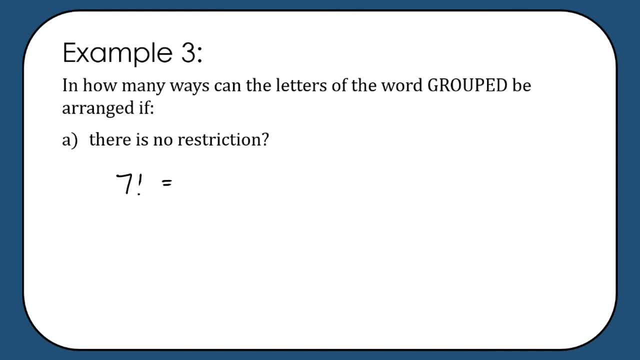 different ways we can arrange them. So 5,040 different arrangements. In how many ways can the letters of the word grouped be arranged if the letters P and D must be next to each other? Okay, so what we've got happening here is: 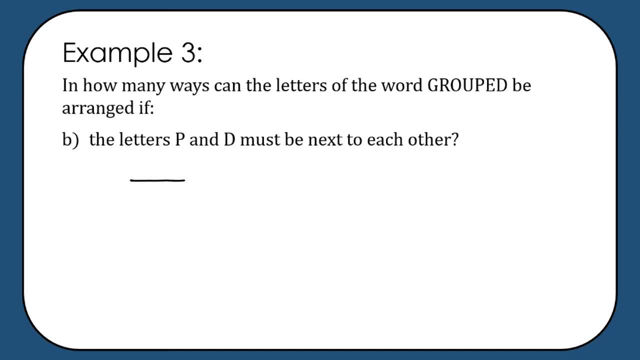 we have to have the P and D next to each other. So we've sort of got two letters grouped together And there are two different ways we could arrange those, or two factorial, such as two. So then the other five letters need to be arranged around here. 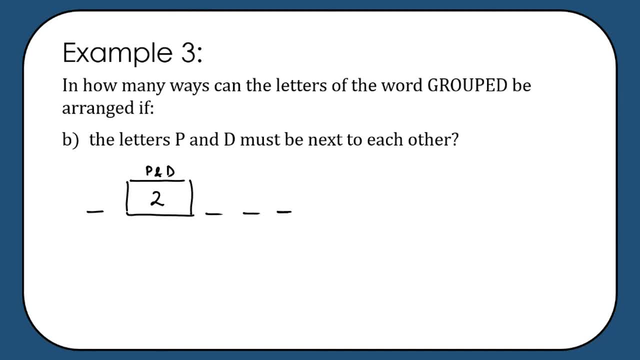 So some of them might be at the beginning, some of them might be afterwards. So what we essentially have here is we're grouping the P and D together- and there are two different ways that they can be arranged- And then treating the P and D as one entity. 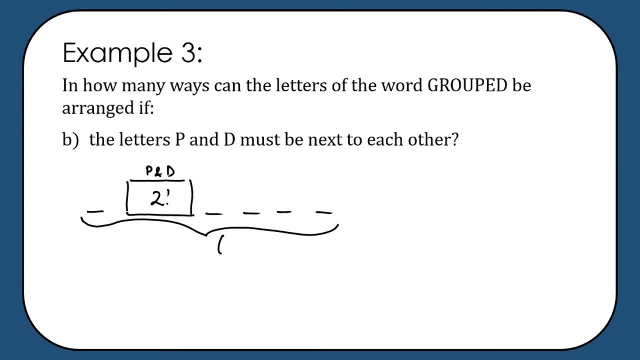 we now have one, two, three, four, five, six things to be arranged. The group with P D in it and the other five letters can all be arranged in six factorial different ways, And then for each of those six factorial different arrangements: 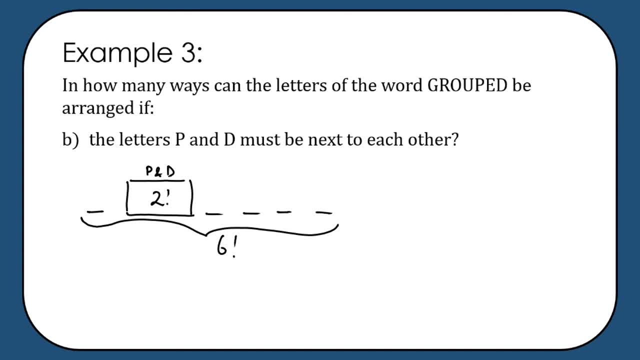 there are two different options, because we could have P and then D, or D and then P within that. So the total number of arrangements is two factorial times six. factorial, which is two times seven. twenty, which is fourteen forty. In how many ways can the letters of the word grouped be arranged? 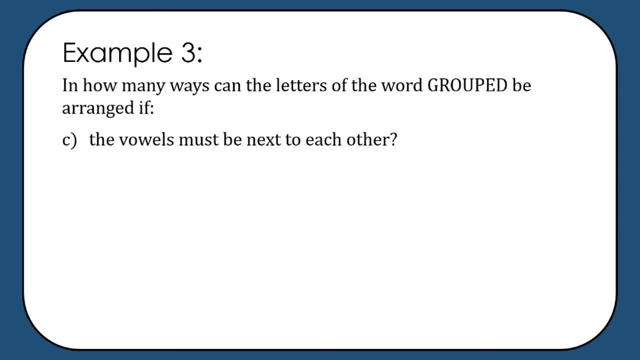 if the vowels must be next to each other. So this is essentially the same problem as before. We have three vowels in this word, so we're going to group those three vowels together And there are three factorial different ways the vowels can be arranged. 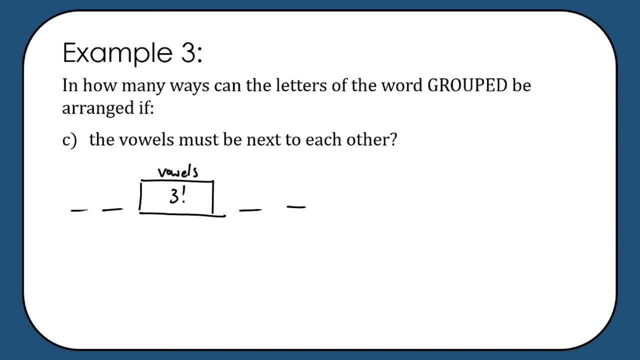 And then we have four other letters around them, or you know, after or before them. So then we need to think about how many different ways can we arrange those five things, which is five factorial, So we're going to have five factorial times seven. 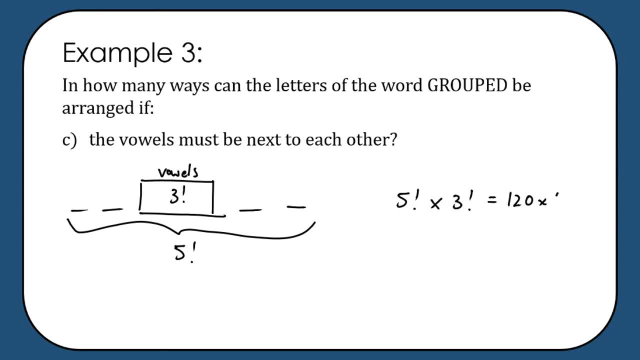 which is three factorial, which is one twenty times six, so seven hundred and twenty. In how many ways can the letters of the word grouped be arranged if the letters P and D must not be next to each other? Okay, so this is where it's useful that we've already worked out. 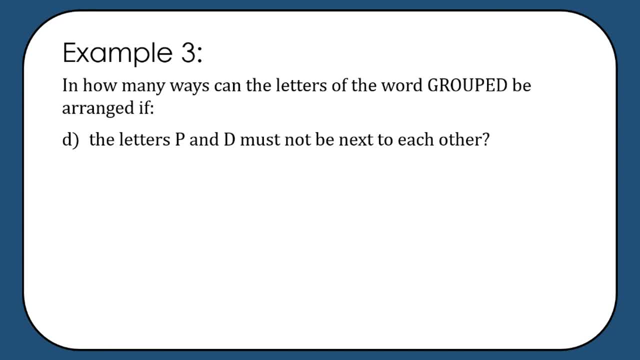 And in fact, even if I was given this question without having been asked part B, I would probably still, you know, find how many different ways can I do it with P and D grouped together and then subtract that from the total number of arrangements. 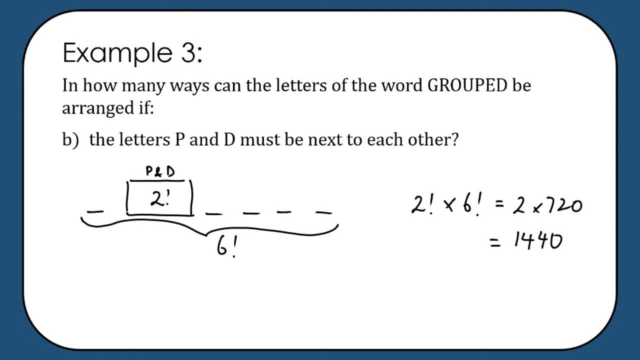 So we know, let's flip back to our previous parts. in part A, we worked out that there are five thousand and forty different arrangements, and in part B, we worked out that fourteen hundred and forty of those arrangements have P and D together. So that means that we need the total number of arrangements. 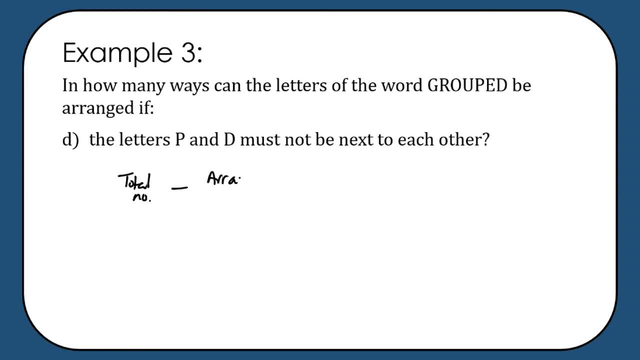 minus the arrangements with P and D together, And so that was five thousand and forty minus one four four O, which gives us three thousand six hundred different arrangements where P and D are not next to each other. So third, last part of this question. 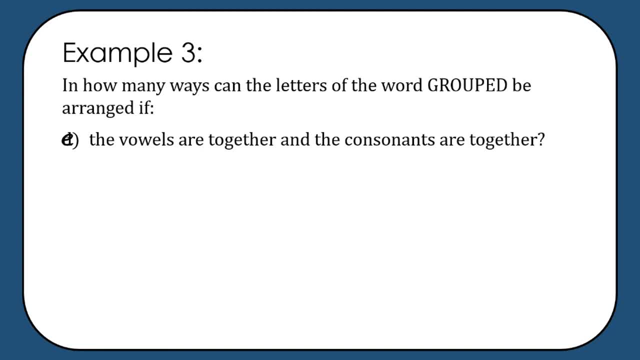 in how many ways it should be part E, apologies. in how many ways can the letters of the word grouped be arranged if the vowels are together and the consonants sit together? Okay, so previously in part C, when we looked at having the vowels together,